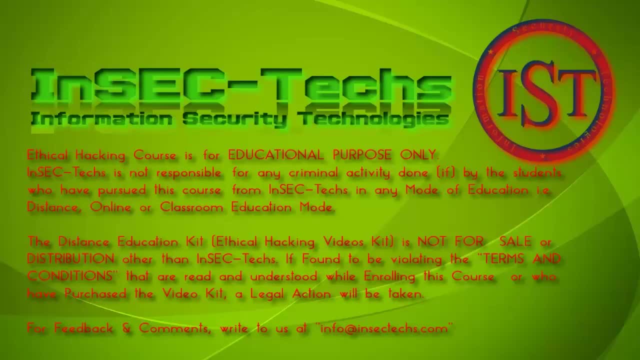 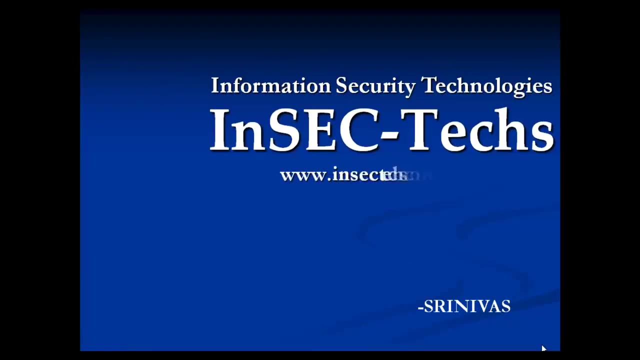 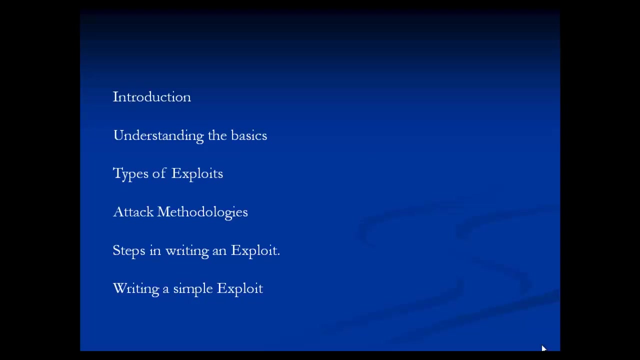 Welcome to Insectex Ethical Hacking course videos- Module: Buffer Overflow and Exploit Writing. In this video we will go through the basics of buffer overflows and exploit writing. We will start from the very basics and we will try to understand what are the exploits types. 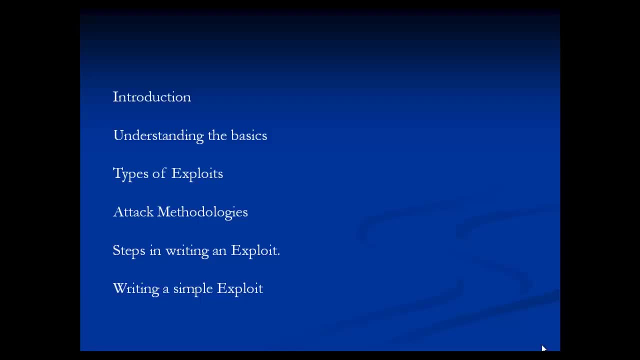 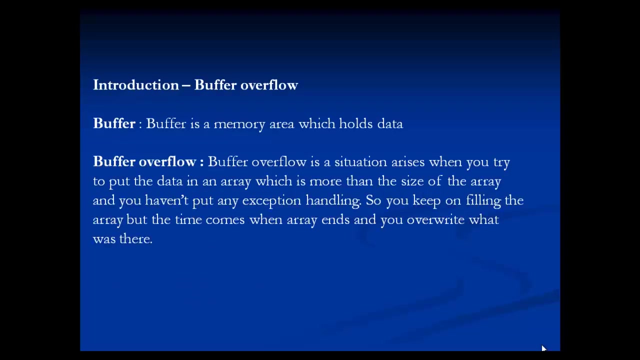 and what are the attack methodologies and what are the steps involved in writing an exploit. And finally, we will try to exploit a simple buffer overflow vulnerability by writing our own exploits. To start with, what is a buffer overflow vulnerability? Before understanding buffer overflow vulnerability, let us try to understand what is a buffer. 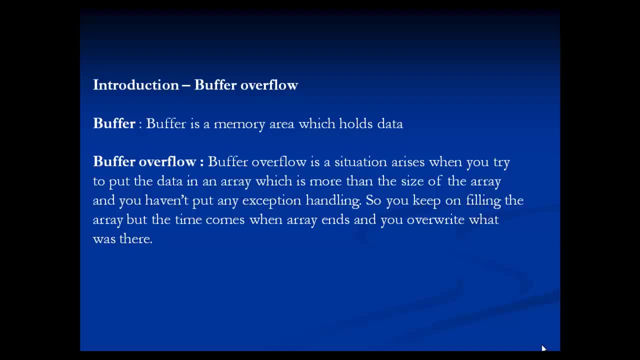 Buffer is a small memory area which holds some data. When we accept some data into this buffer which is out of a limit, It overflows and this is called buffer overflow. So buffer overflow is a situation arises when you try to put the data in an array which 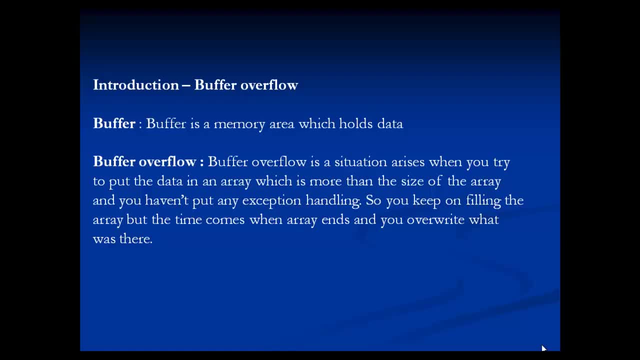 is more than the size of the array and we haven't put any exception handling. So we keep on filling the array, but the time comes when array ends, you overwrite that what was there and we will see what it is exactly using a live example. 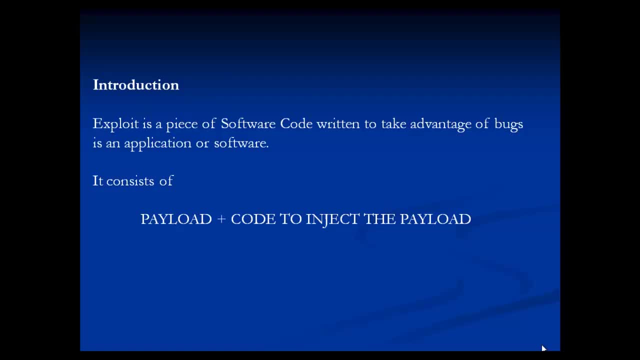 And exploit is a piece of software that takes advantage of a bug in an application or a software. Let us say we have a buffer overflow vulnerability. Now we will write a simple exploit to take the advantage of that buffer overflow vulnerability. And this is a simple piece of code and this is called exploit. 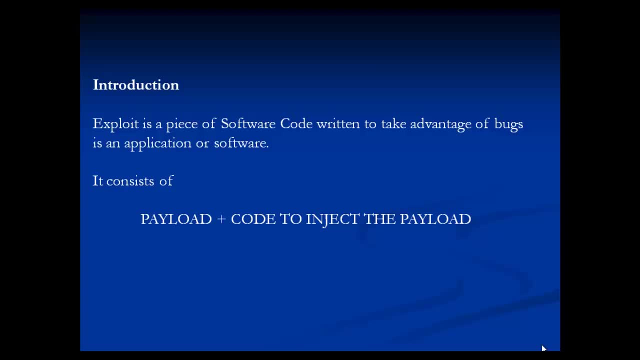 And this exploit consists of two things: One is payload and another one is code to inject. And this exploit consists of two things: One is payload and another one is code to inject. And this exploit consists of two things: One is payload and another one is code to inject. 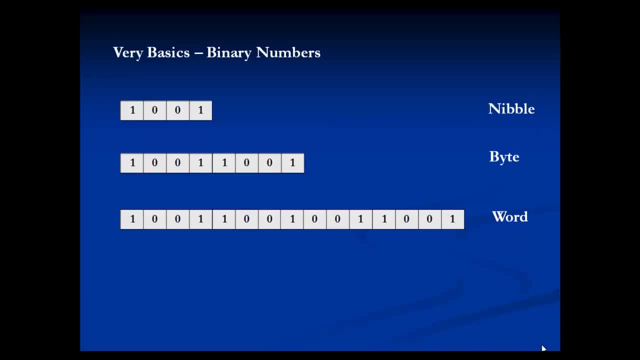 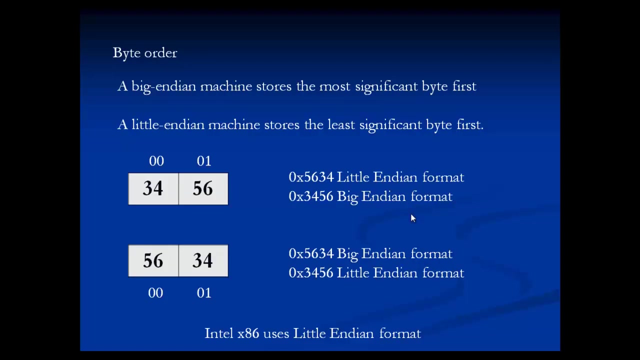 eigen Sauber to inject the payload into the vulnerable application. Now to start with the very basics: Stanford Server and eight bits is called a byte. two bytes is called a word. now what is the order of a byte? byte order or indianness generally. 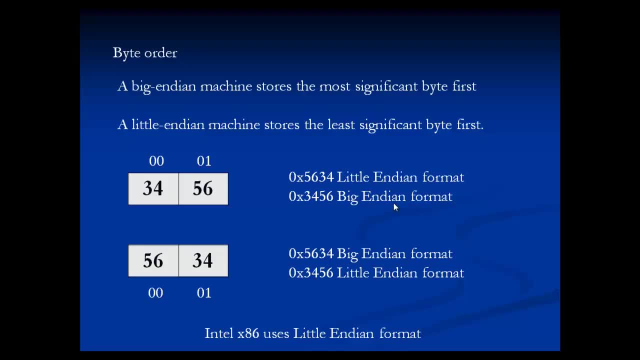 machines take two types of byte orders. one is big indian format and another one is lil indian format. generally, big indian machine stores the most significant byte first. for example, in this example 34 is one byte and 56 is another byte, and if it is in big indian format, 34 is the most. 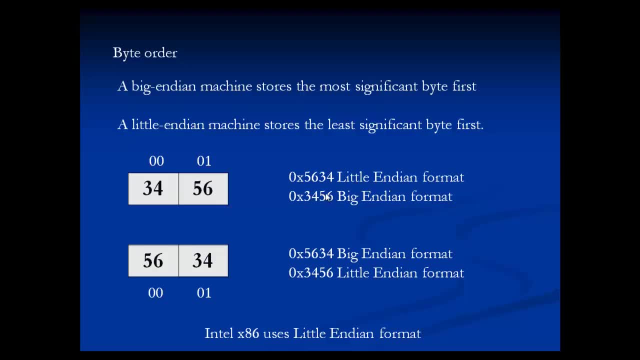 significant byte, so we have kept it first. and 56 is the least significant byte, so we have kept it at the end. so this is big indian format. the same thing in lilindian format is the least byte will be kept first and then, and the most significant byte will be kept at the last. so this is lilindian format. 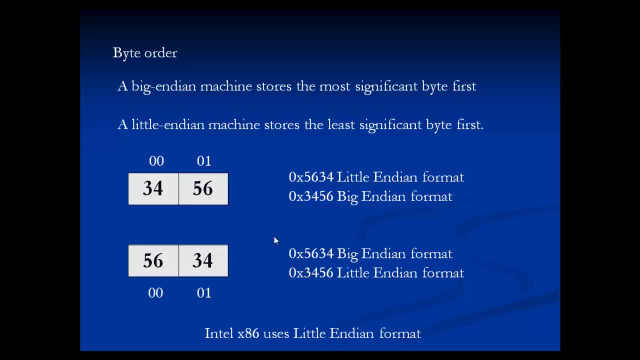 this is a representation of bytes, and similarly in another we have another example where we have taken 56- 34. we have just reversed the previous example, so in this case lilindian format will become 0x3456 and big indian format will become 0x56 and 34, and in our examples we are using intel cross 86 architecture, so we use lil indian. 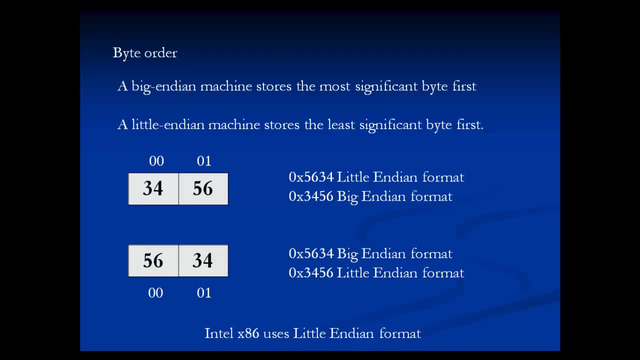 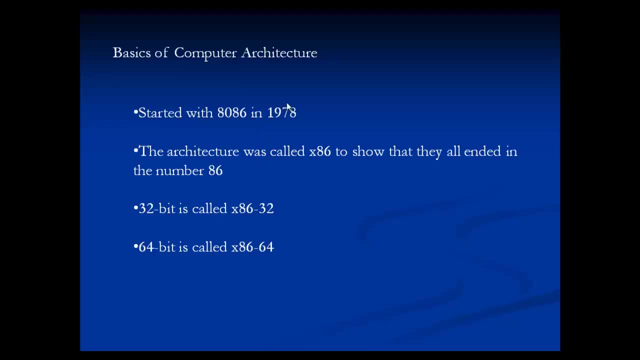 format throughout the examples. so let us try to understand the basics of computer architecture cross. we have started with 8086 processors. in 1978 it's cross 86 architecture, the computer architecture, and was called cross 86 to show that they all ended in the number 86. 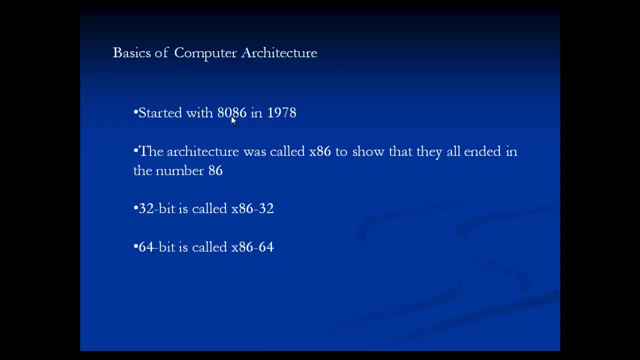 and we used to have 32-bit processors and those are called cross 86- 32. this is the representation for 32-bit processors and for 64-bit processors. this is the representation cross 86 and 64.. and the basic difference between 32-bit and 64-bit processor is: 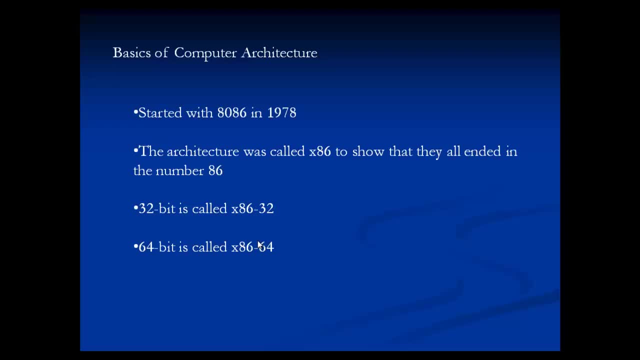 the register. before understanding the difference between these two, we need to understand what is a register. a register is a small amount of storage used by the cpu, where the cpu keeps the data it needs to access the quickest in order for optimum computer performance. now let us understand the bits. the bit designation: 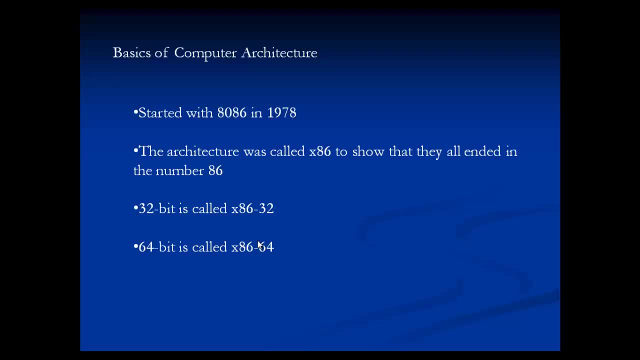 refers to the width of the register. it means it is a. if it is a 32-bit register, it holds more than a 16-bit register and an 8-bit register. similarly, if it is a 64-bit register, it can hold more data than a 32-bit register. so this is the width of the register. 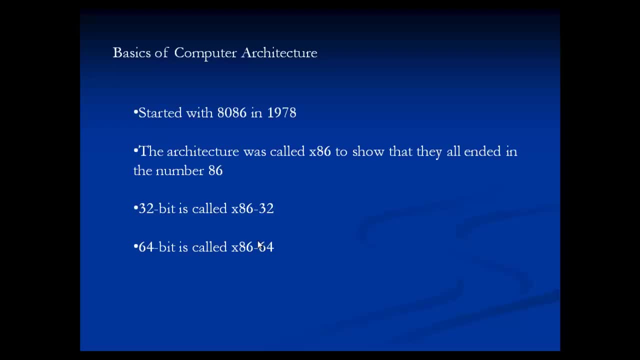 the number- the understand i mean the bits 32 and 64- entitles the width of the register. so the the more ample the space in the cpus register system, the more it can handle, especially in terms of utilizing the system memory. now a cpu with 32-bit register can have a selling of. 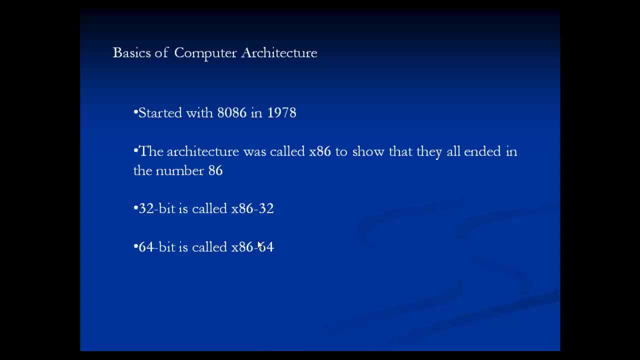 2 power 32 registers addresses within the register. this is equivalent to four gigabytes, hence it cannot support more than 4 gb of ram, whereas in the case of 64-bit register, the register is able to bit registers. it can have 2 power 64 addresses within the registers, which is very huge. now, 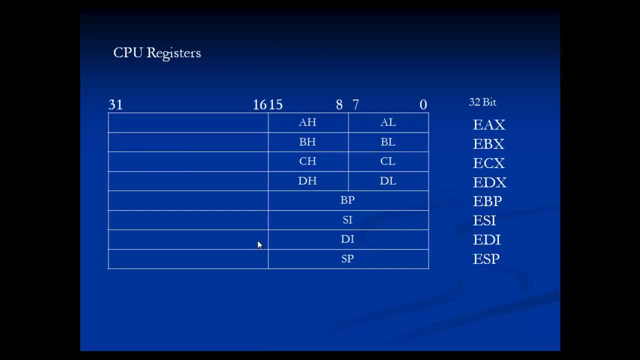 let us try to understand the cpu registers. we have in 32-bit architecture, 1, 2, 3, 4, 5, 6, 7, 8 registers, and another one is eip that we haven't included here, which is instruction pointer. now, EAX is the accumulator register, which is used to store the results of our calculations and this: 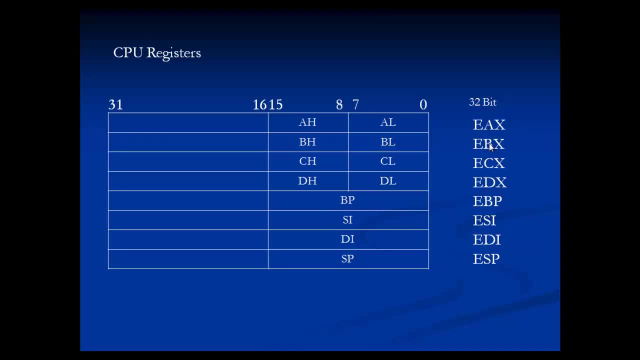 EBX register is not designed for anything specific, but it is completely free for extra storage space, and ECX is the count register this use. this is a universal loop counter. it functions similar to a variable we use to set up loop counters, loop counter value and this. EDX is an extension to the accumulator and it is 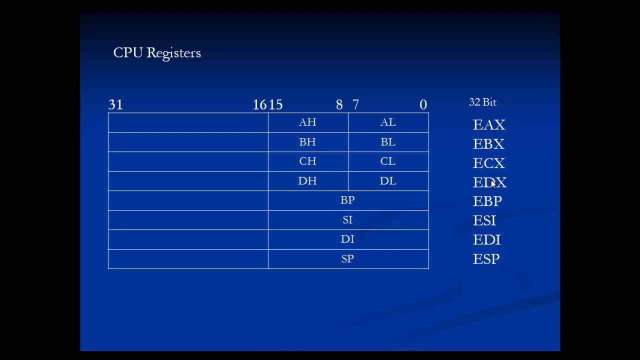 useful for storing data related to the accumulators- current location. and then we have EBP. EBP stores parameters or variables on the stack. the base pointer holds the location of the current stack frame. we'll see what it is. the full form of EVP is extended base point of. I got to tell EAX stands for extended. 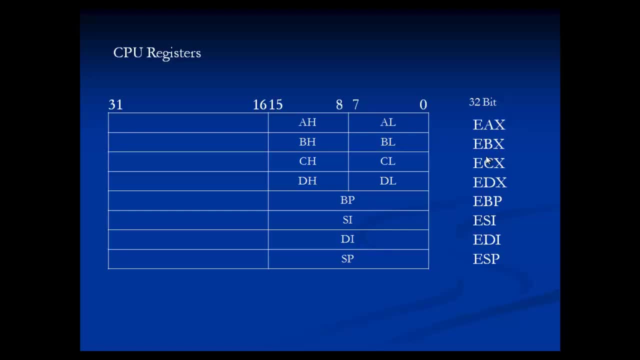 accumulator register and EBX stands for extended base register and ECX for counter register, EDX for data register, ebp for extended base pointer. now e, e, e, e, ESI. it holds the location of the input data stream. Whatever the input we are taking, the registers are taking, the processor is taking, it holds the location of that input data stream. 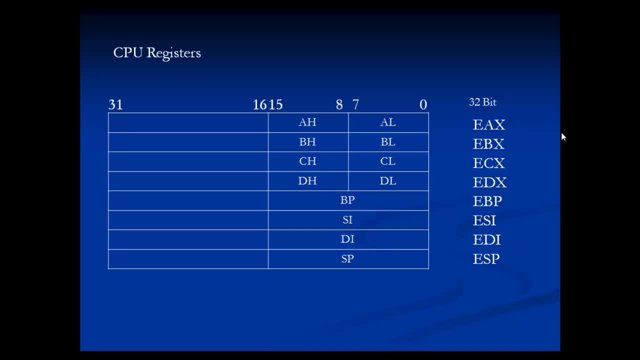 Now EDI. EDI points to the location where the result of a data operation is stored. In other words, every loop must store its results somewhere and this destination index points to that place. And finally, we have ESP. it is the stack pointer. it always points to the top of the stack. 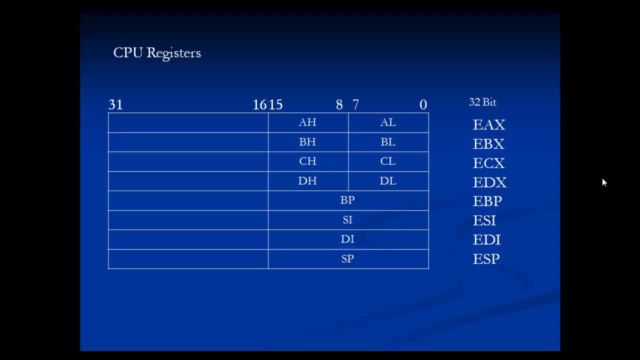 We will see couple of registers among these registers. in couple of other slides We will try to have a deeper understanding of what these registers do. And now, when a register is referred to by its extended name, it means you can see here we have removed E in this EAX. 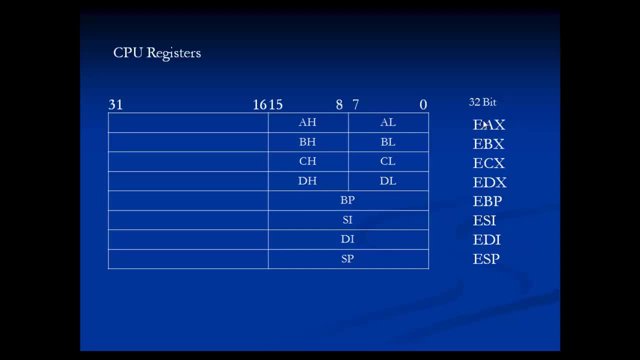 So we are in this 32-bit architecture, 32-bit register. we are using E as an extra one, So when a register is referred to by its extended name, it indicates that all the 32 bits of the register are being addressed. 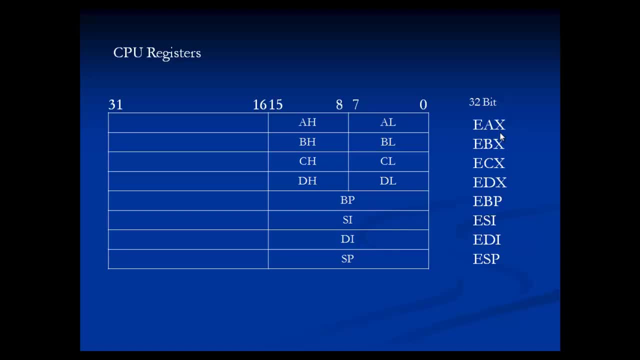 And these registers can be broken And the first 16 bits of each register can be referenced by simply removing the E from the name You can see here. this is the AH which is broken. EAX has been broken into AH and AL. 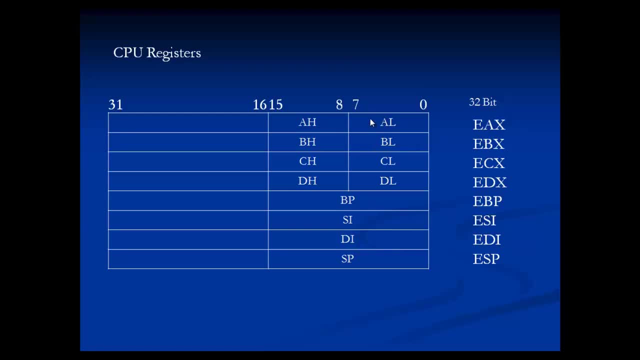 Now additionally registers let actually we have. just we can just remove this EA E from this EAX And we can represent It as EAX for the first 16 bits. Now this EAX in turn can be broken into AH and AL. 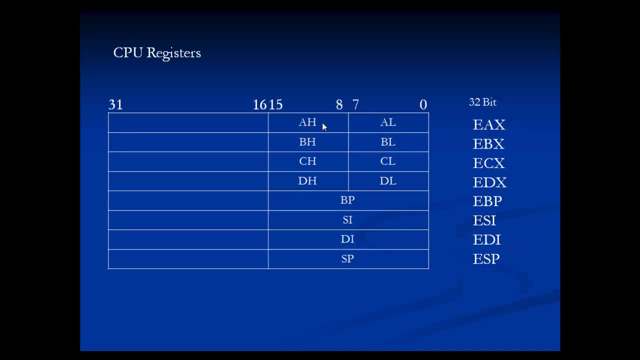 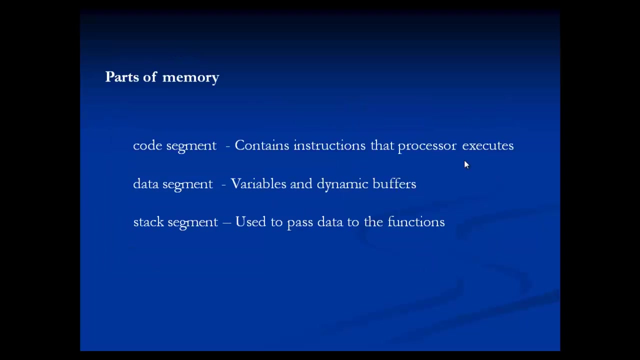 0 to 7 AL and 8 to 15 AH. This AL stands for lower addresses and AH stands for higher addresses. Similarly, the other registers also can be broken into the further subsets of themselves. And Now let us try to understand the parts of the memory. 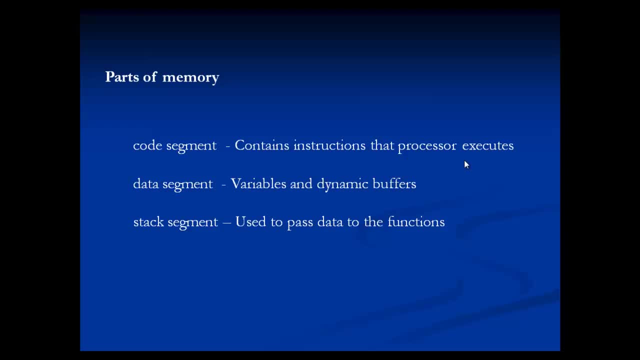 We have three parts in the memory. One is code segment and another one is data segment and another one is stack segment. This code segment contains instructions that the pointer, the processor, executes. It means the actual program instructions that are being executed by the processor. 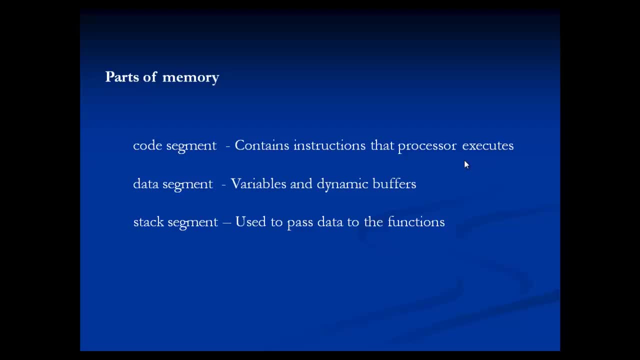 And the data segments consists of variables and the dynamic buffers And, finally, the stack segment consists of the. it is actually used for passing the data to the functions. It is very useful. The stack segment is very useful when functions are getting called. 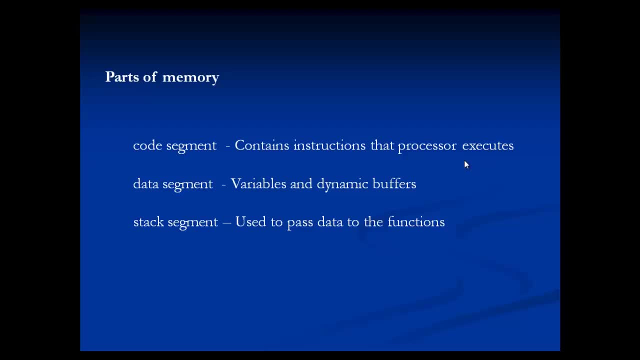 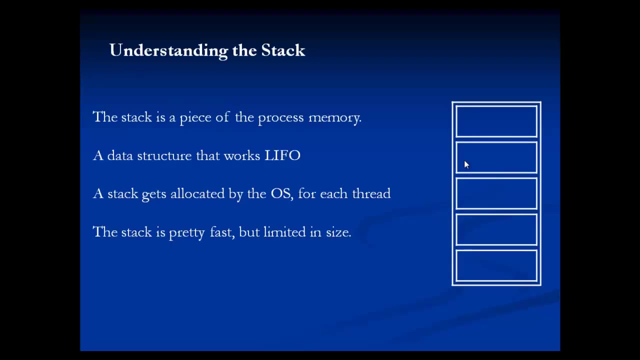 We'll see the. we'll see an example of how it works: the stack segment. But to understand the stack, The stack is a piece of the process memory, It's a data structure that works. LIFO- last in, first out- We'll see what it is. 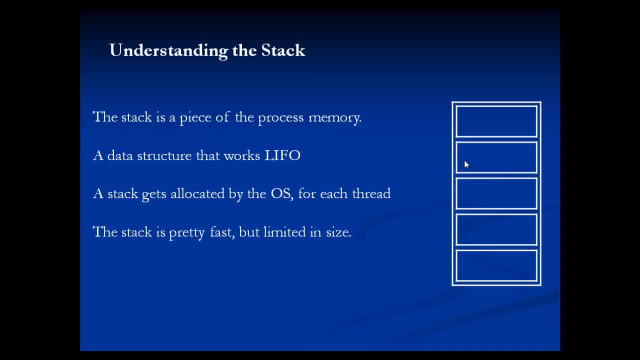 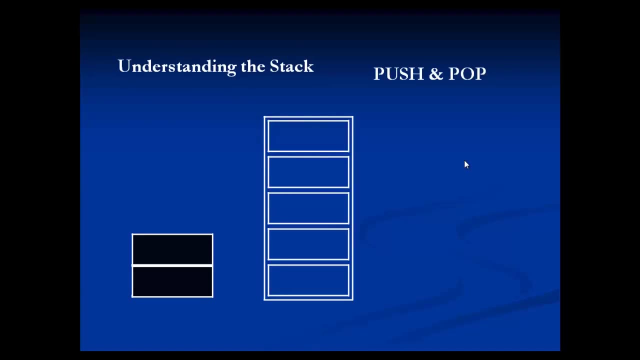 And a stack gets allocated by the operating system for each thread And the stack is pretty fast but limited in size. Whenever a function is called, a limited amount of size will be allocated for a stack by the operating system. Now, If you go further to understand, 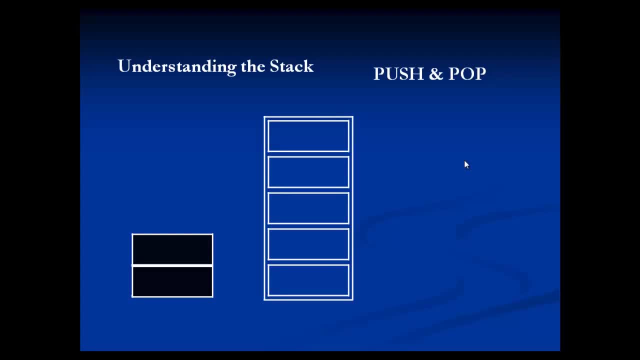 The stack. there are two operations which are very, very important on a stack. One is push and another one is pop. Whenever we try to push, a element will be attached, added to the top of the stack. Now we have no elements in the stack and this will be the top location of the stack. 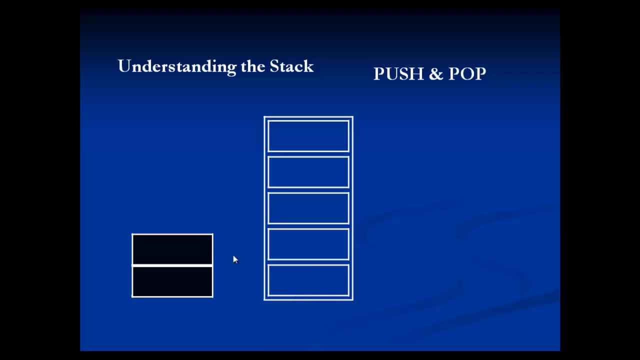 So if we try to push some element onto the stack, The element will be pushed into this location, And this is how it happens Now. we have this location as the top of the stack. So if we try to push some other element onto the stack, 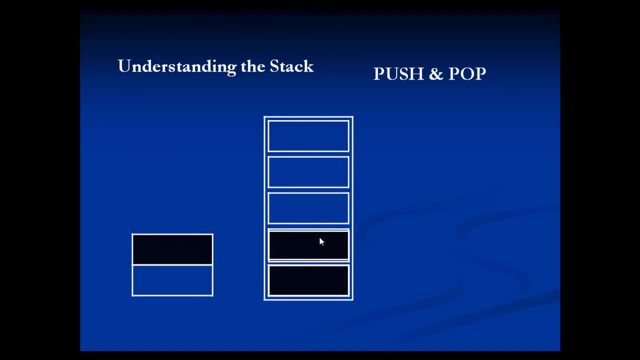 Element will be pushed onto this location. So, similarly, we can push one more element onto the top of the stack. So every time we try to push, us push an element, it will be pushed onto the top of the stack. Simply, in other words, pushing is adding elements to your stack onto the top of the location. 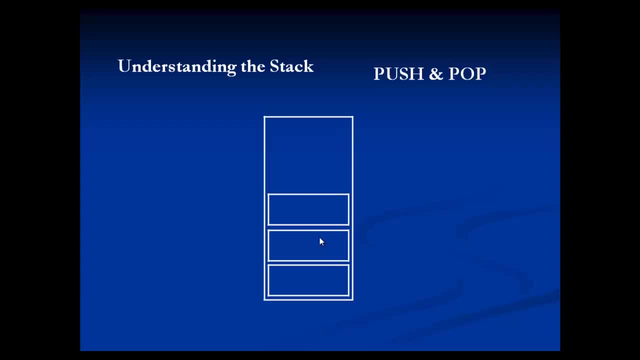 Now we have one more operation, that is the pop. pop will remove One item from the top of the stack and it puts in a register. it means if you try to pop the element from the top of the stack, it will be removed. 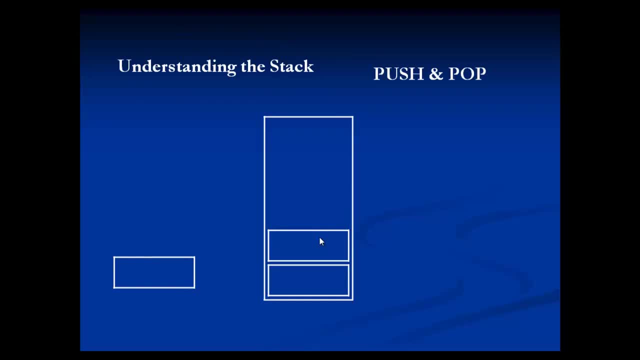 Like this: And if you try to pop one more element, it will be popped out from the top of the stack, from the top of the stack, like this. so this is how pop operation works. now let us try to understand what is stack pointer. stack pointer will always point. 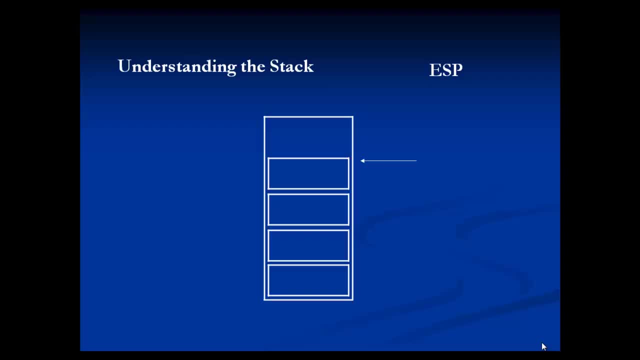 to the top of the stack. it means if you try to delete one element from the stack, currently the stack pointer is pointing to the top of the stack, which is the top element. now, if you delete this, if you pop this particular top element like this, now the stack pointer will point, will be pointing to the top of the 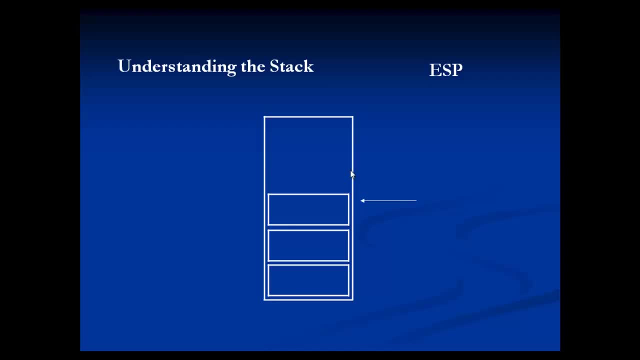 element. this is how a stack pointer works. and now let us try to understand the stack further. whenever a function is entered, it means, let us say, function a is calling function B, now we have. function a is calling function b, now we have. function a is calling function b, now we have. 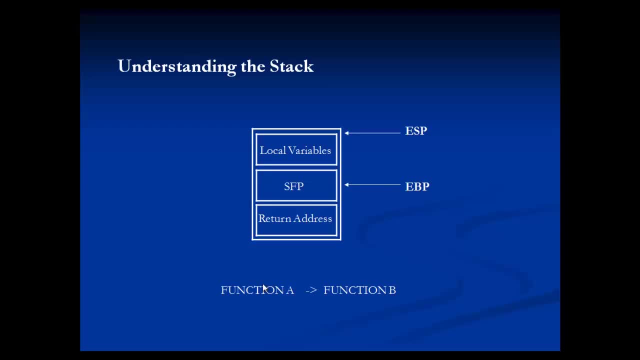 entered into a function. now a stack frame in is created. this is just some information on the stack and that is filled in an filled in and organized. when function a calls function B, a stack frame is pushed on to the stack. a stack frame consists of stack frame pointer, which is SFP, and return address. this is: 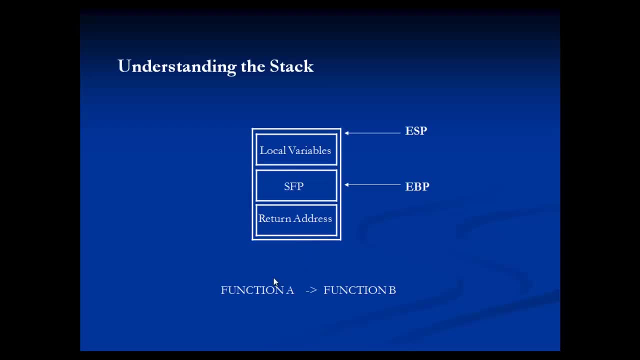 the location of the next instruction in function a, because function a has made a call to function b. after completing the execution of this function b, it has to go back to function a. it has to execute the next instruction, and address of that next instruction will be stored in this written address. now. SFP holds. 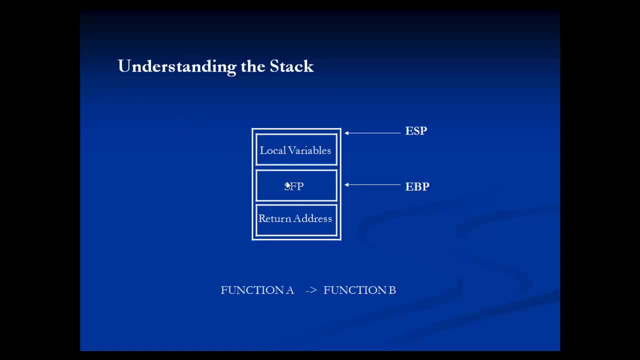 this stack frame pointer holds the location of function ace SFP. it means the function is stack frame pointer and the location of the current stack frame pointer will be stored in a register called EBP extended base pointer. To be clear, when function A calls function B, it first pushes the address. 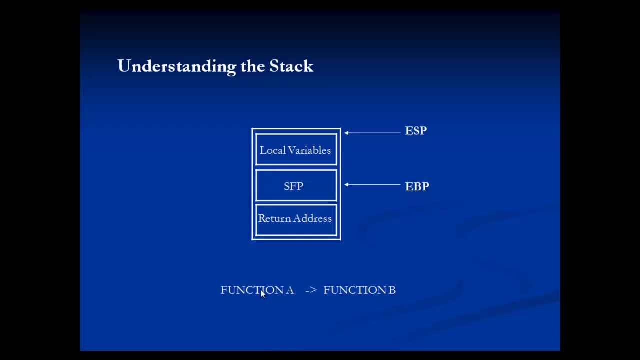 of the instruction. after this function call, This becomes function B's written address. Now function A pushes the location of its own saved frame pointer. Now stack frame is almost complete, and then it jumps to function B. Now, whatever the code is, 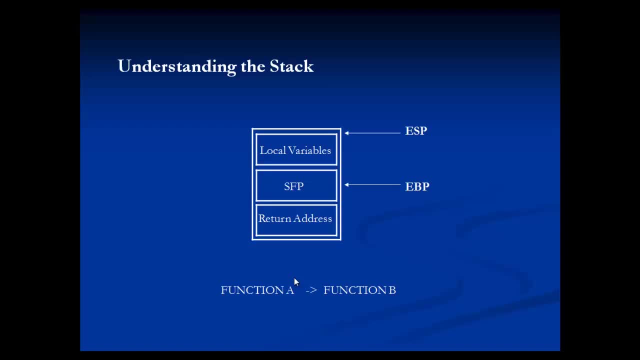 there in function B, it will be executed. When it is done, it will go back to function A, And this is what a stack frame pointer is. Now let us try to understand some basic assembly instructions, which are very useful. The first one is push EAX. 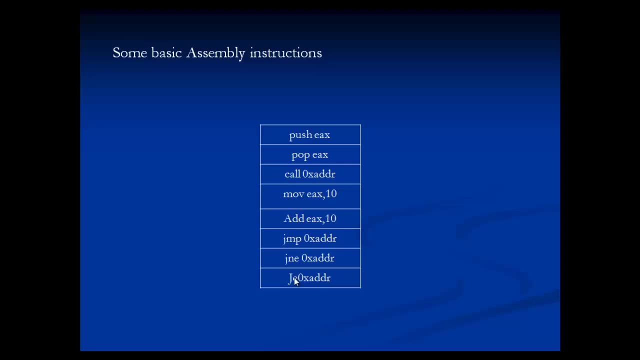 This will push the EAX value onto the stack, its accumulators value. Now pop EAX. It will pop the value of EAX from the stack to a register. Now call some address. This particular instruction will make a call to a function at this particular location, which is 0xADDR. 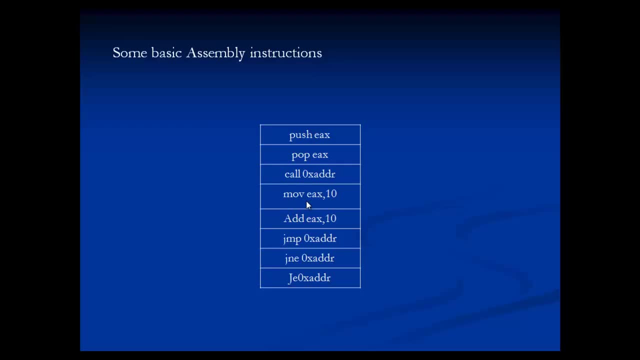 it is the address Now: move EAX 10.. This particular instruction will move this value 10 into accumulator register Add EAX. What this does is it will add the value 10 to the value of EAX register and it will save it in EAX. 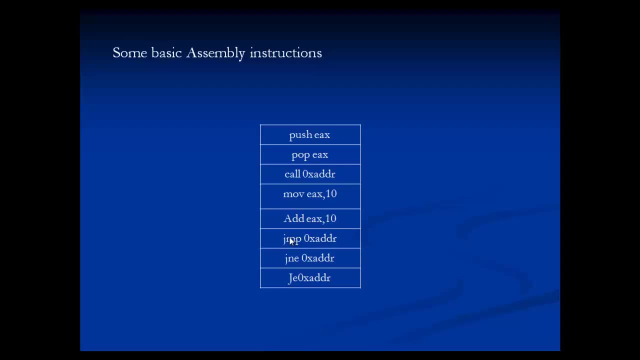 now the next instruction is: jump some specific address. what it does is it will jump the flow to a specific address and the next one is j n e jump. if not equal, it will try to compare some results, and if they are not equal, then it will try to jump to the some specific instruction. 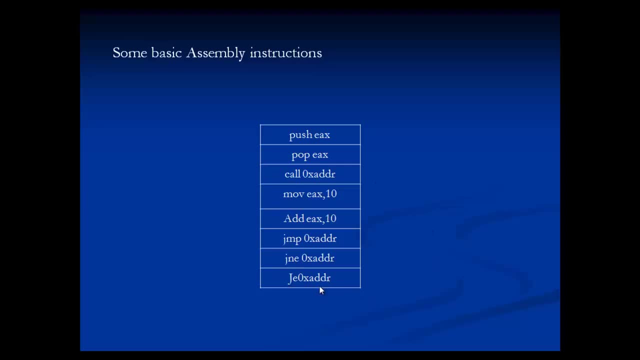 similarly, if the comparison is equal, it will. it will try to jump to a specific instruction and these instructions are just to give a brief understanding of how assembly instructions work. but it will not give the complete understanding of assembly language. so you have to try to understand assembly language by following some resources on internet or somewhere else. 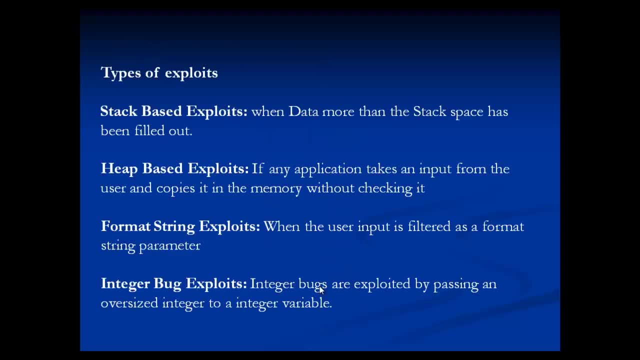 so i'm just moving on to the next slide. let us try to understand what are the types of exceptions exploits we have now. now, the first one is stack based exploits. when data more than the stack space has been filled out, then that type of exploits are called stack based exploits to be more clear. 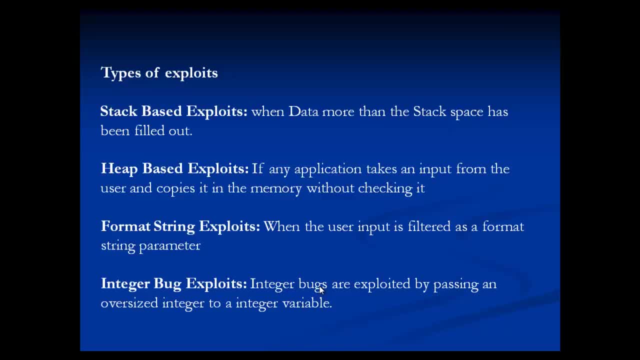 it exploits the stack based buffer overflow. when data more than the stack space has been filled out, this kind of attacks occur. attacks attackers may manage to push some malicious code onto the stack which may redirect the flow of the program and execute the malicious program which the attacker wants to execute. we will try. 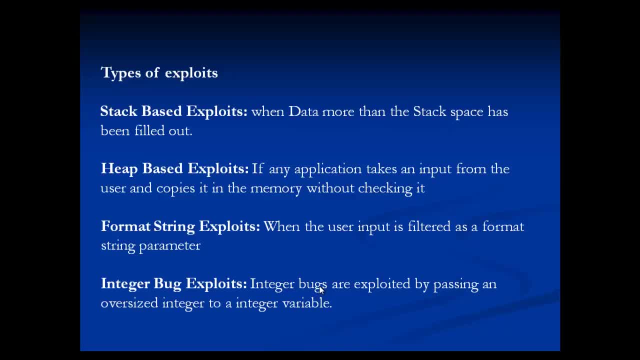 to. we will try to see an example of this particular stack based buffer overflow later in this video, and the next one is heap based exploits. heap stores the data which is dynamically created with the functions such as malloc and all the other functions such as this and all if any application takes an input from user and copies it in the memory without checking. 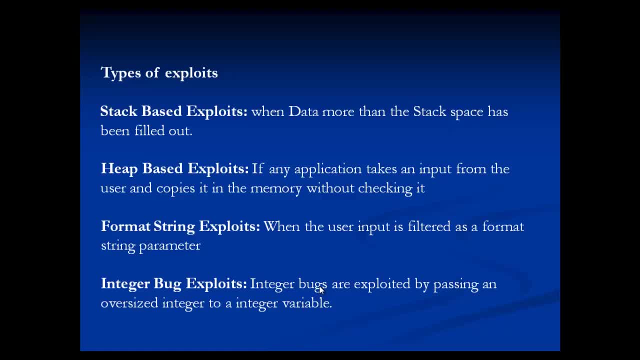 it, a heap overflow may occur. it can cause a serious damage, resulting in compromising the entire application, and the system itself is a system as well. and the next one is format string exploits. this can be used to crash a software or to execute a malicious code. when the user input is filtered as a format string parameter, this attack may occur. functions in c. 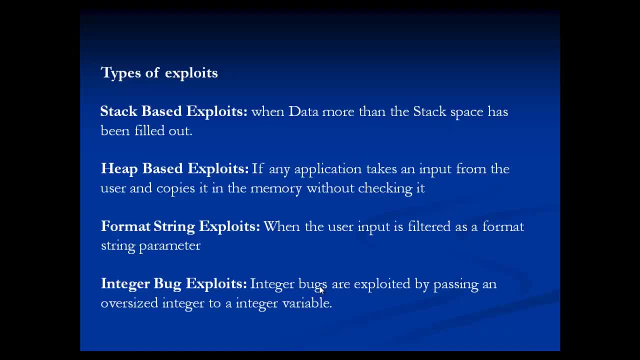 such as printf, uses format tokens such as percentile s, percentile x to print data from the stack or possibly other locations in memory, for example printf. this kind of format string parameters may cause format string exploitations. and the next one is integer bug exploits. integer bug explo. integer bugs are exploited by passing an. 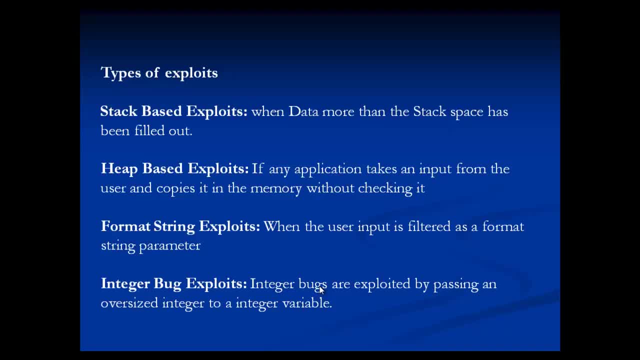 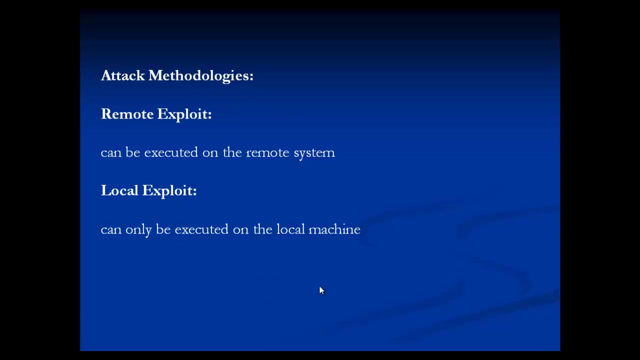 oversized integer to a integer variable. it may cause overwriting of valid program control data, resulting in execution of malicious codes. and this is very brief about the technology types of exploits. we have lot more. we have to go and we have to explore them. and now let us try to understand the attack methodologies. the one is remote. 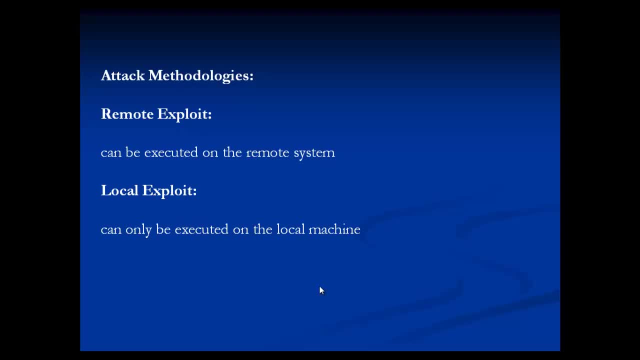 exploit and another one is local exploit. remote exploits can be executed on the remote system. these tend to exploit the services running on the remote system to gain access to that system, for example, an FTP server taking malicious input from a client machine, resulting into a buffer overflow attack. these are called. 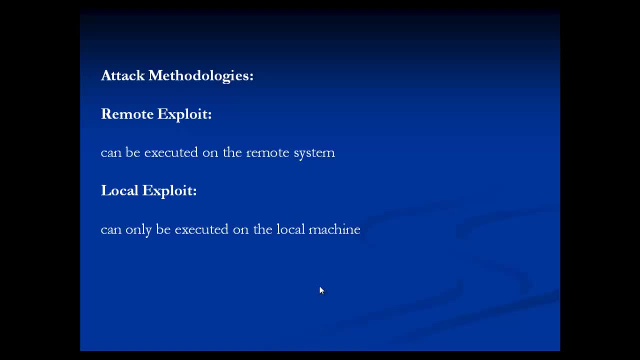 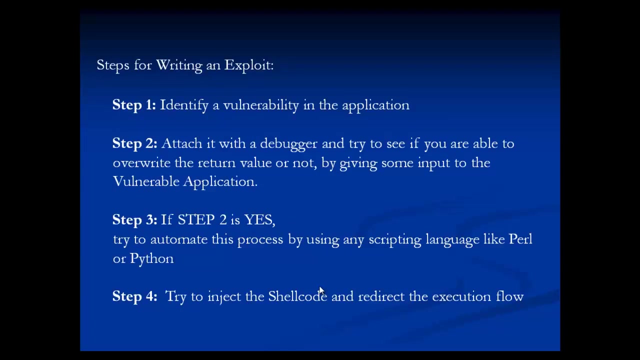 remote exploits and only let us try to understand local exploit. this can be executed on the local machine where the vulnerability has been found and cannot be mutated to a remote exploit privilege escalation attacks are often done because of this: local exploits. now let us try to understand the local exploit. and what is the local exploit and what is the? 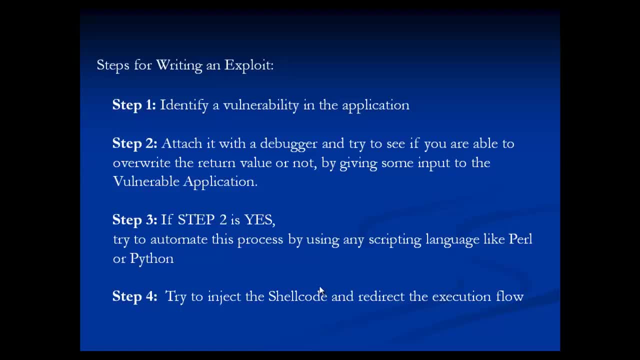 understand the steps. in writing. a simple exploit. first, we need to identify a vulnerability in the application and we have to attach it with a debugger and try to see if you are able to overwrite the return value or not. it means the EIP instruction pointer. by giving some input to the 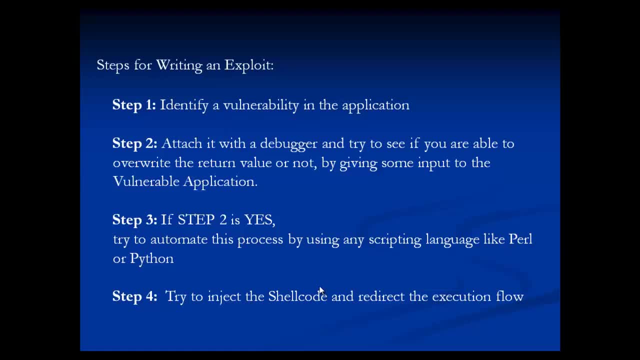 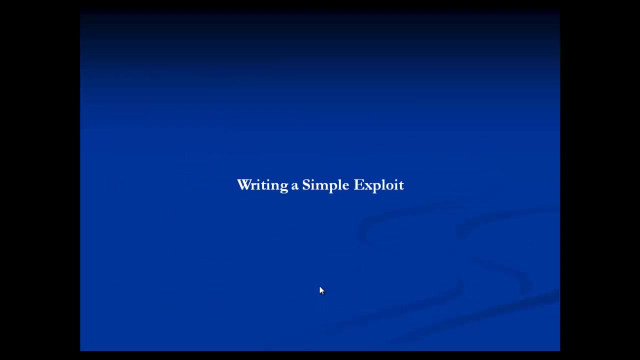 vulnerable application. and step 3 is: if step 2 is yes, then try to automate the process by using any scripting language like pearl or Python. and then the last step is: we have to try to inject some shellcode and redirect the execution flow. and now let us try to understand these these steps in a practical way. so 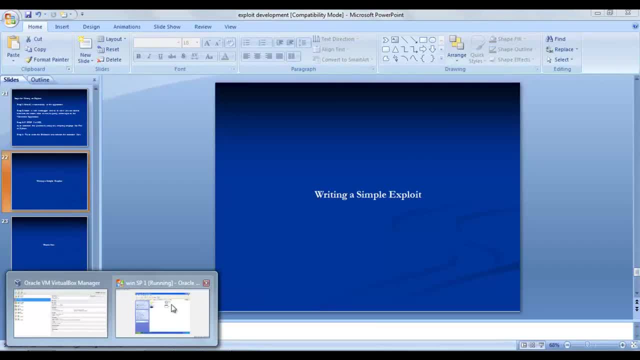 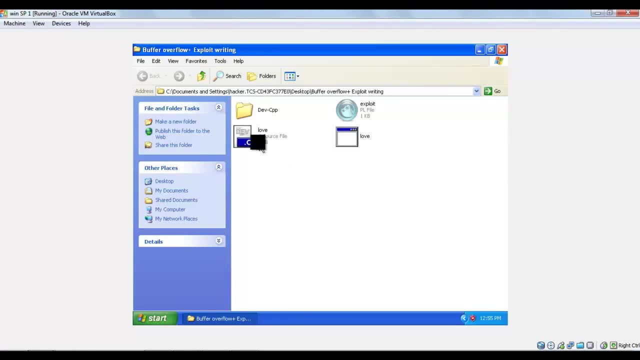 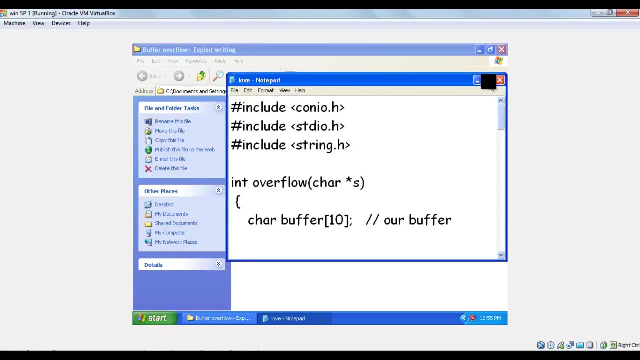 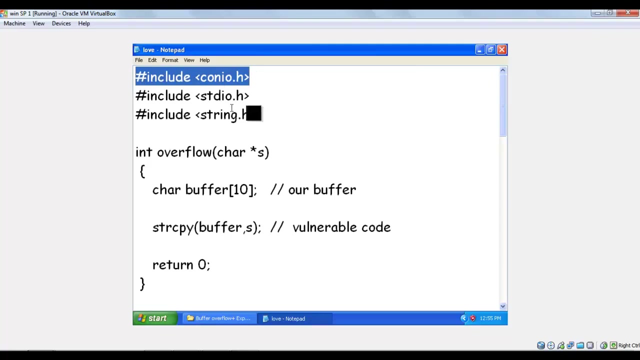 let us try to write a simple exploit which exploits a buffer overflow vulnerability. and now, in this example, I am just going to take a very simple program. let us see the source code of the program. it is a very simple C program. we are taking hash. include SDI or dot H, cornea dot H and string dot H. after then, 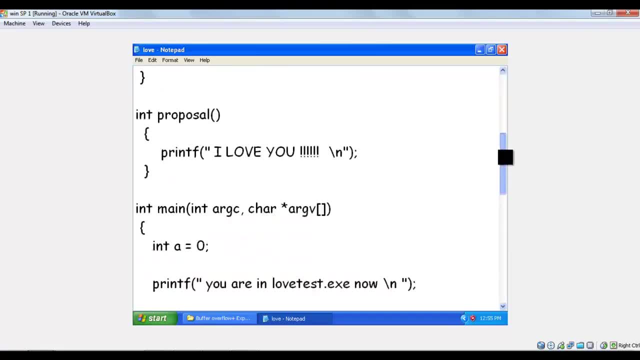 it will move on to the main function and let us see what it is doing. the main function is taking some arguments from the command line and it is assigning the value 0 to a and immediately it is printing some statement. you are in loudest: dot exe now. 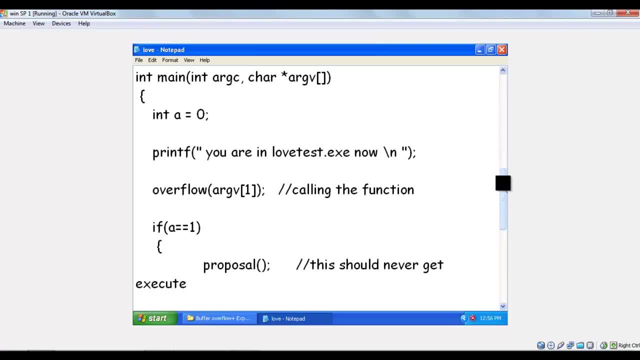 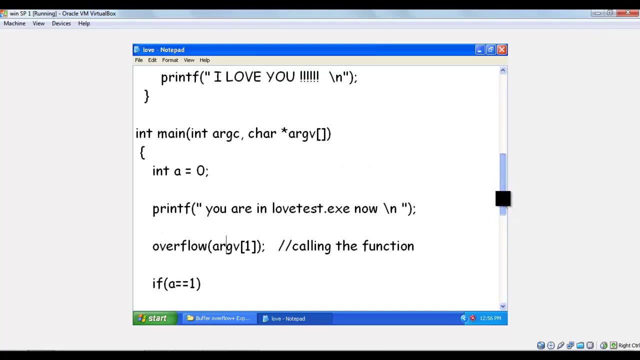 this is a very good example. this is a very good example program if you really want to propose a girl using your technology hacking. so the next function is overflow off and it is actually calling the function overflow off with the argument argv of 1. now it's taking the definition. it will go to the overflow function definition. let 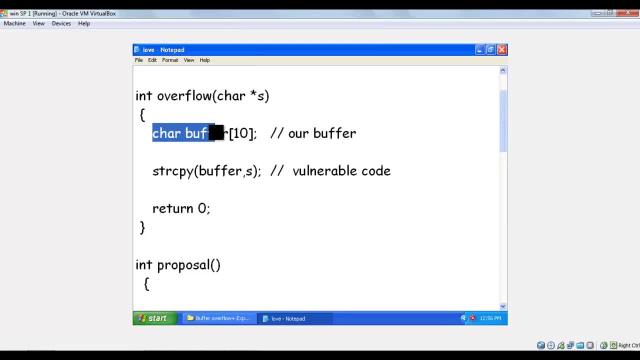 us see what happens, and this is what is being happened: it is taking the argument and it is putting into the buffer which actually accepting 10 characters. now, after then it is copying into a variable min, a buffer, and after then it is returning 0, and this is the vulnerable code which is having no bound checking. 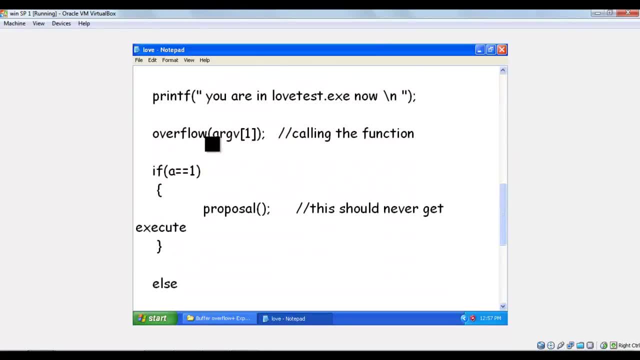 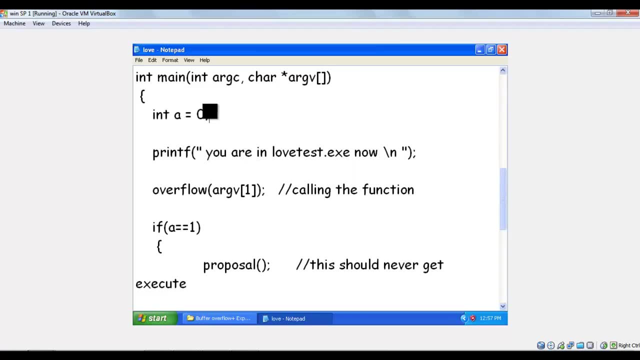 function and it is checking if a equals to 1 and if you observe, a is already assigned with the value 0 and it will never will become 1.. So it will never go into this particular if block and this proposal of function will never be executed. and let us try to understand what happens if this. 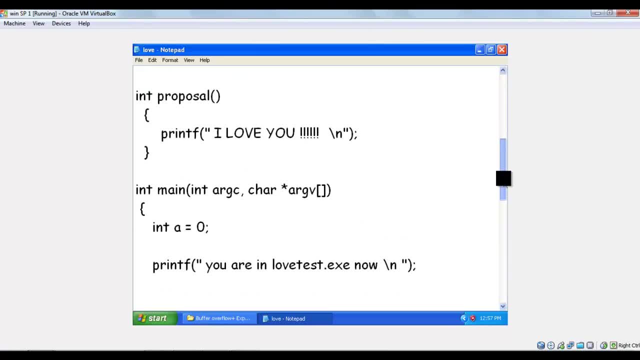 proposal of function executes. Also, it is printing. I love you, but unfortunately this proposal of function will never get executed and it is our job to make it execute, and that is what we are going to do in this particular demonstration. and if it does not work, if a equals to 1 does, 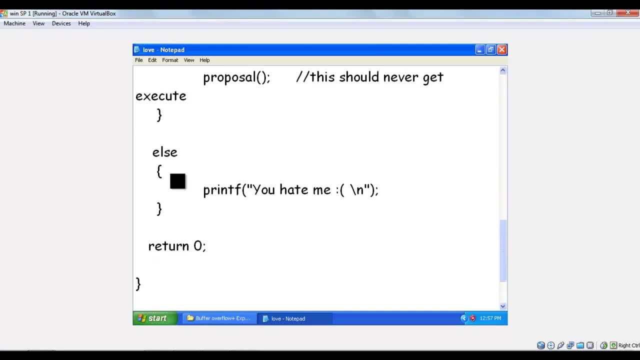 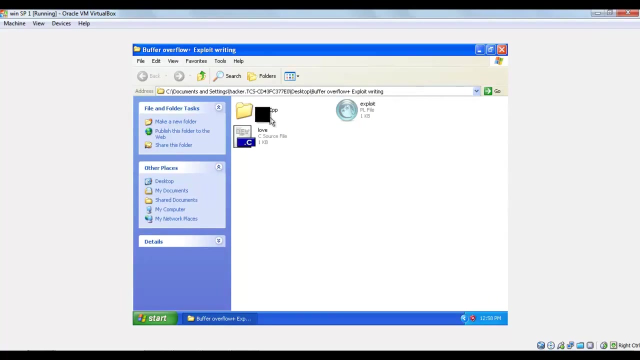 not happen, it will print: you hate me. It means your proposal will fail. So let us try to give this code to Dev C++ application- I am just copying it- or else close this. I am just deleting this function. I mean exe file I have already created. Now let me open this with: 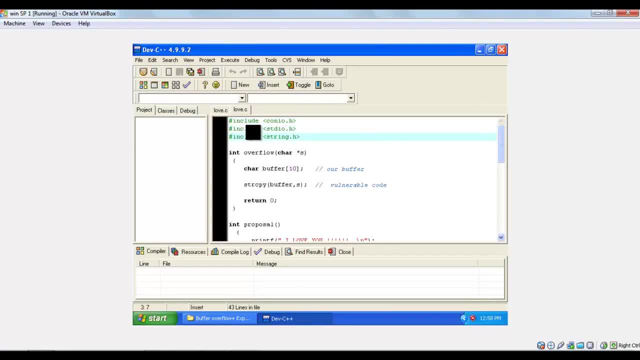 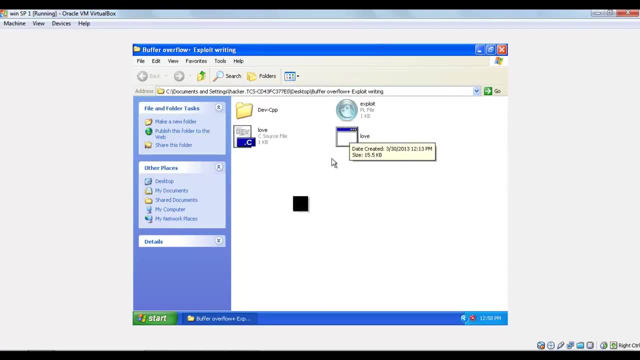 Dev C++ and the same function. Let us try to compile it. Close it If you try to observe the same location. a new file, loveexe, has been created. Now let us try to execute using a command line. Just go to this path, copy this and paste it. 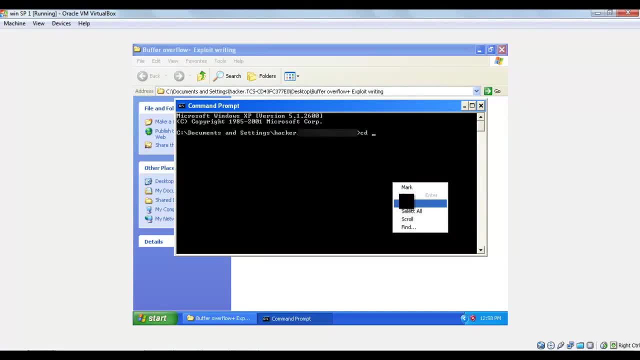 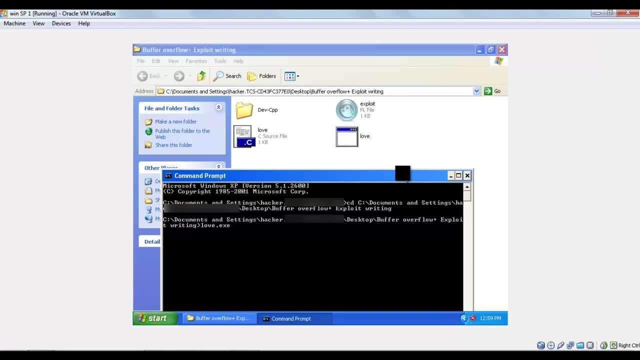 All right, Now we are in the current look and now let us try to give some data. Now, let us try to give some data. Now, let us try to give some data. It is actually taking 10 characters, and if we give more than 10 characters, the application will be crashed. 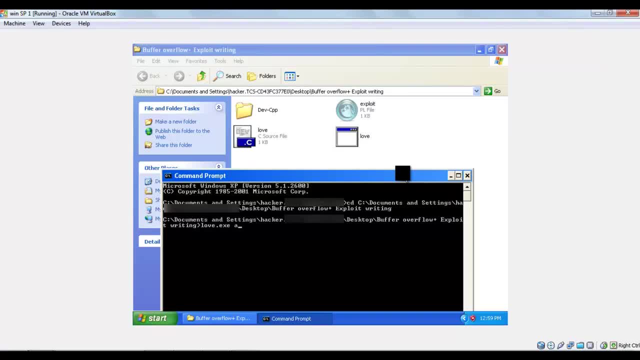 It is actually taking 10 characters and if we give more than 10 characters, the application will be crashed. Let us try to understand what it is: Abcdefgh, which is less than 10.. It is printing: you hate me, and that is obviously right result. 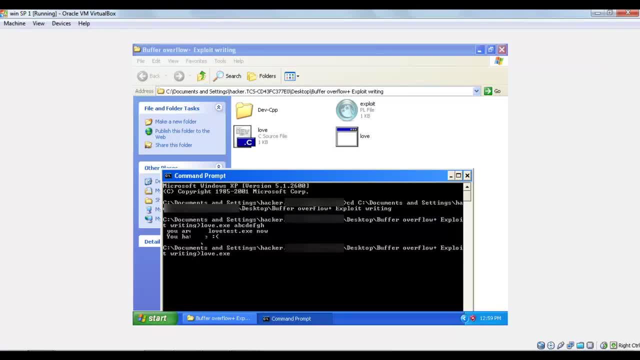 Let us try to give some random input which is more than 10.. I am just going to give some 20 to 30 characters: abcdefgh, i, j, k, l, m, n, o, p, q r s, t, u, v, w, x, y, z, and now a, b, c, d, e, f, g, h, i, j, k, l, m, n, o, p, q r s t. 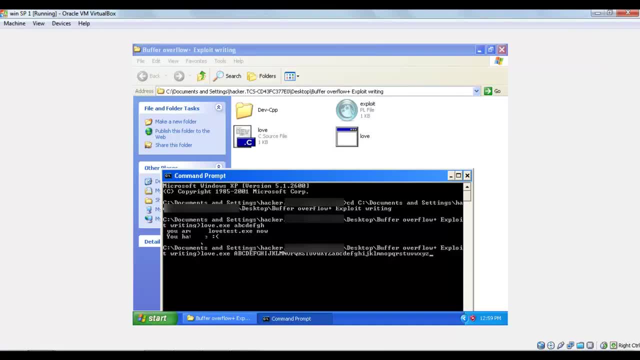 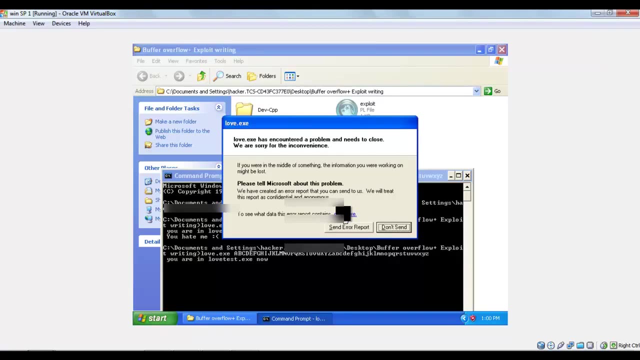 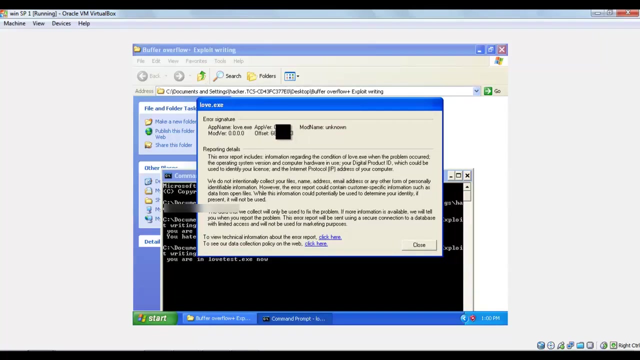 u, v, w, x, y, z. we have given 52 characters, which is more than 10 now if we press enter. awesome, the application got crashed. now let us try to understand what's happening by just clicking. click here: great, it is showing offset 66, 64, 64 and 63, and this is. 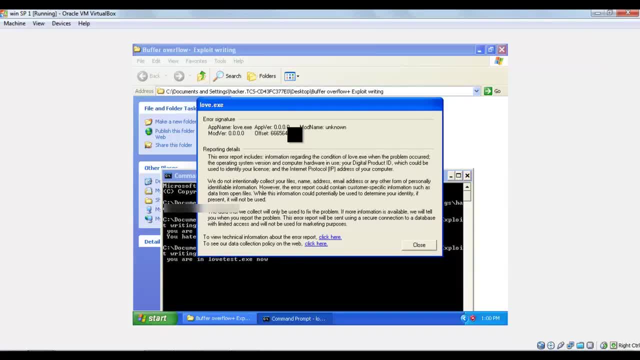 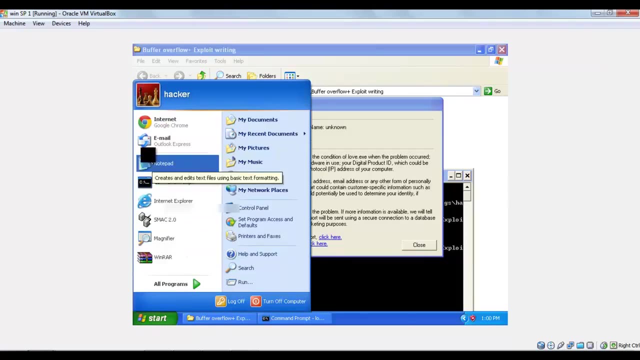 the value of eip. the next instruction to be executed. we are actually filling the buffer and we are redirecting it to this particular address, and this 63, 64, 65, 66 is. i'm just copying it and pasting it in the notepad. let me close this application first. 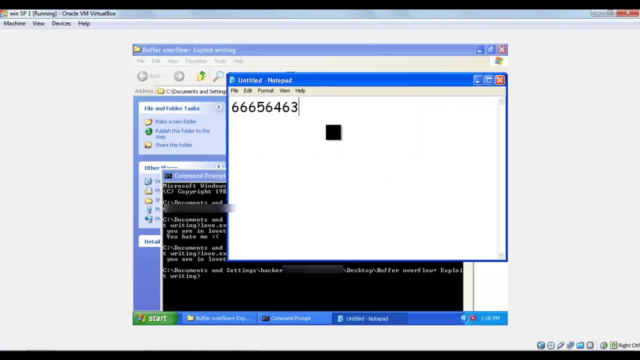 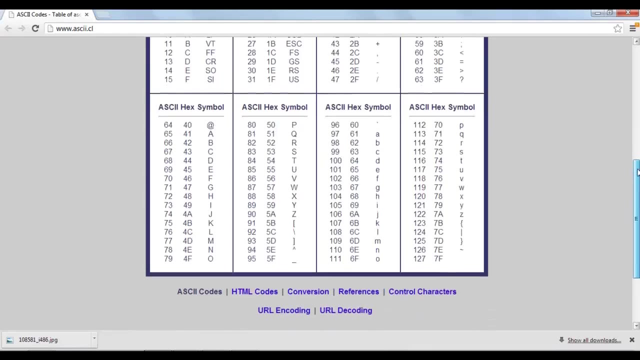 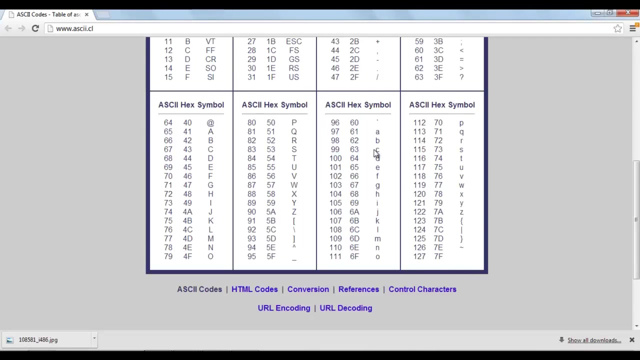 this 63 is. i don't know what it is, so let me just. it is in some format which i cannot understand, so let me go to google and try to understand what it is. it is hex format of the ascii value 99 and which in turn represents small c, so 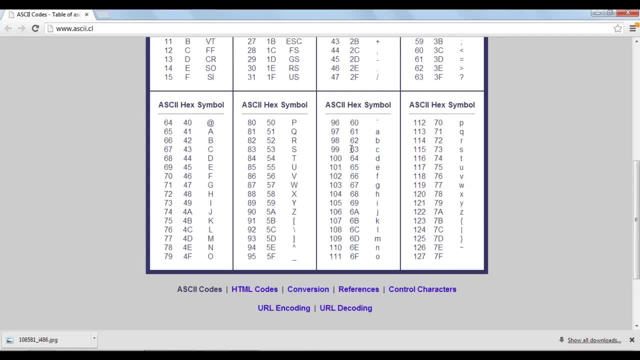 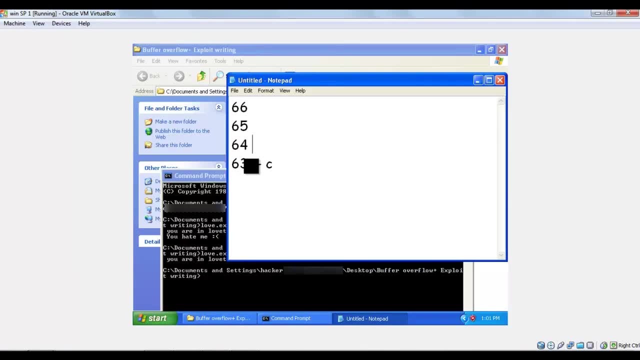 this is the value of small c, which we are actually, which we have actually entered into that application. so this is c and this is the drawing here through which we are actually getting the text schools out as a very nice book by taking: is this right? this is the behavior. view the money mean. so this is all strong and if you are in dollar, that is something you can get. that performance was the particular kind of Germany and this was something there is that a, there was a k, a, a right, so it would be at a real expensive value, which was not the 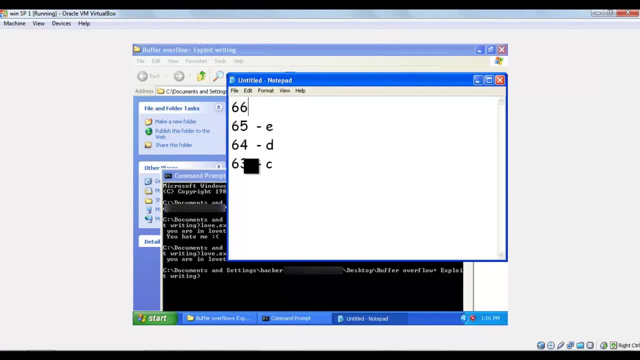 d and this is e and this is f, so we have four characters. this is the address of your eip, but, as we discussed, we are using lelandian format, so it should be like 0x, 6364, 6566. now this is gonna be our address, which is: 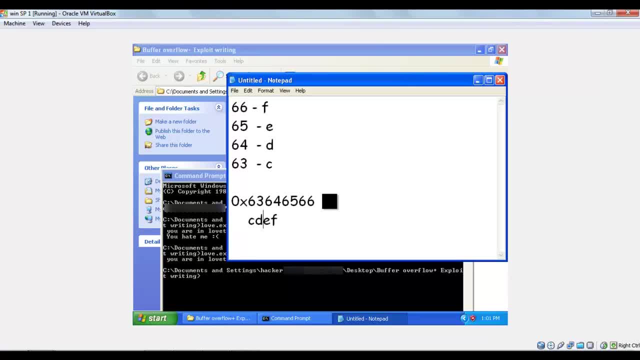 c, d e f. so characters- still a, b, c, d e, f to a b are accepted properly, but when it comes to c, d e f, the buffer is getting overflown and it is the application is getting crashed. so this is what we want. now we are able to find out. 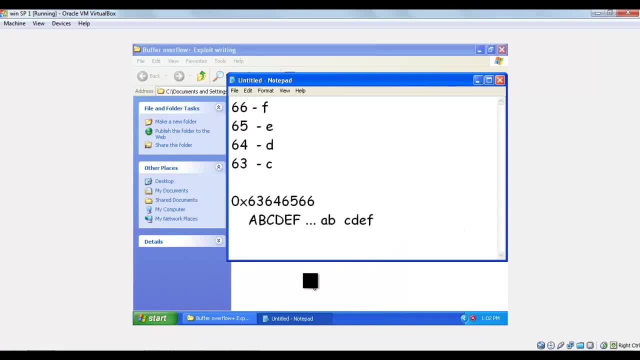 that application is getting crashed by actually loading some eip, some random eip value, into the, into the eip register. now the application doesn't know what to execute, so that's why it is getting crashed. now what we try to do is: we'll try to give. 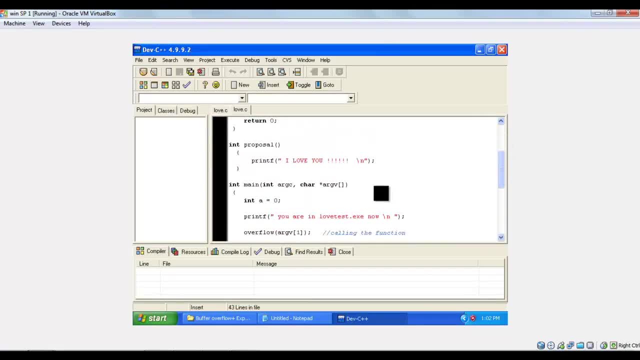 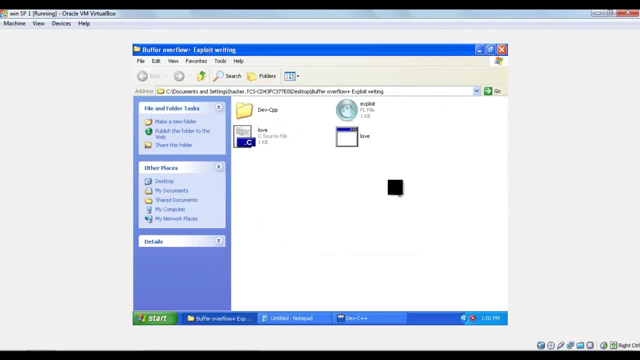 the address of this particular proposal of function so that, instead of getting crashed, even it gets crashed, it will execute this particular proposal of function. that is the idea behind this particular attack. So the buffer is getting overflown, It is vulnerable, It is taking some external EIP value. So, instead of giving some random EIP value, we will give some. 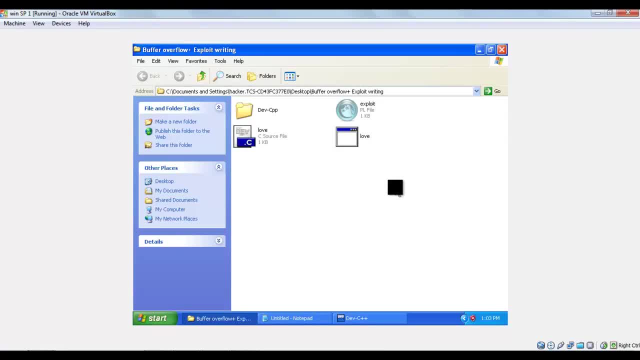 meaningful EIP value. So that is what we are going to do now. But we don't know what is the address of this proposal of function. So let us try to open all edbg. I am just searching for all edbg in my system. 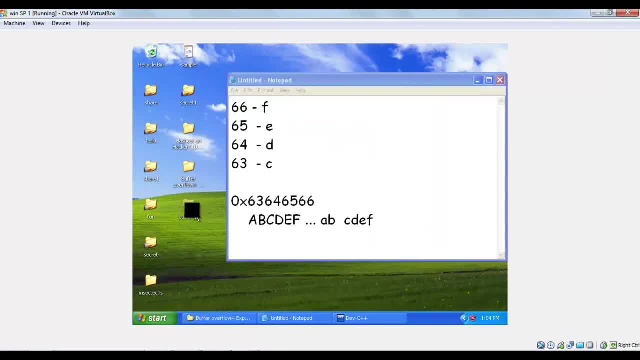 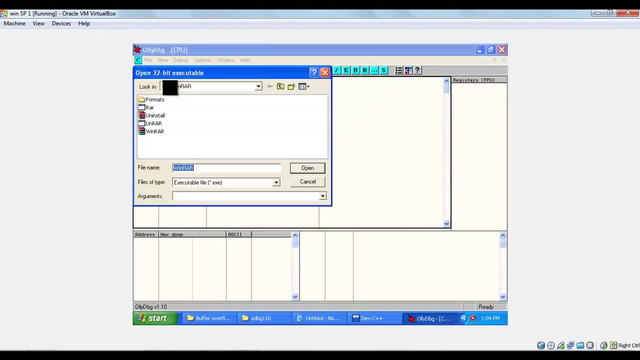 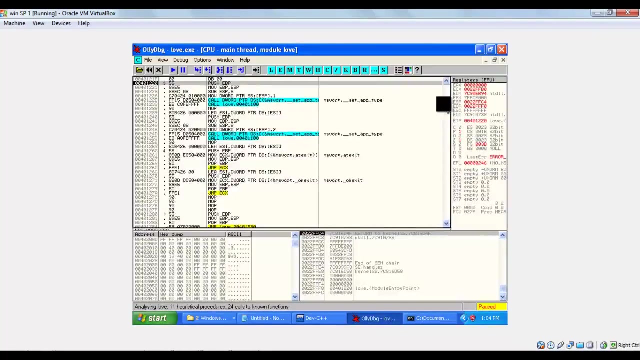 And let me, I got my all edbg here. I am just opening this. Now let me open my low dot exe, which is in my folder. So I am just opening it And you can see if you go down. yes, we got some beautiful message. You are in low dot, low test dot exe. now 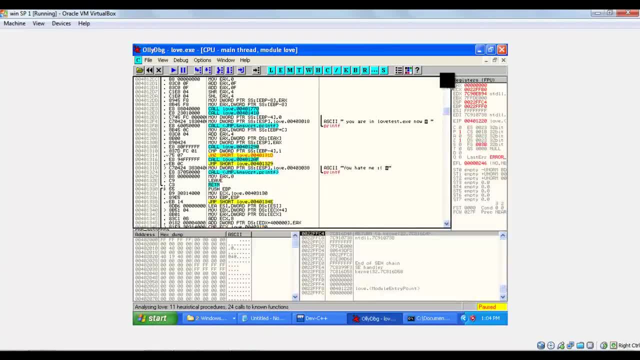 And another one is: you hate me, But we are interested in. I love you And, if you observe, this is: these are the, these are the opcodes, These are the virtual addresses that are being used by this program And these are the assembly instructions that are being converted from the. 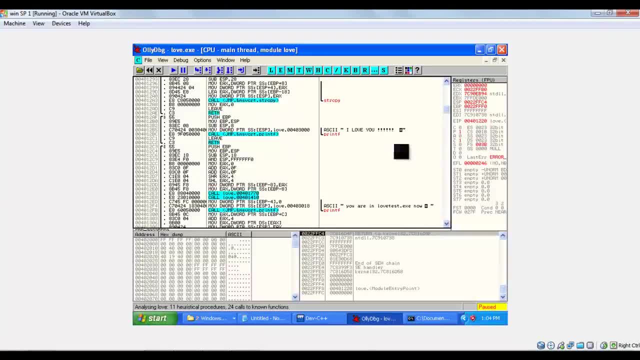 opcodes for human understandable format And these are the comments we have And these are the registers we have seen in our presentation And this is the dump of the opcodes which we, which we can analyze. Now we are interested in this particular. I love you message because we want to display it by executing the program. 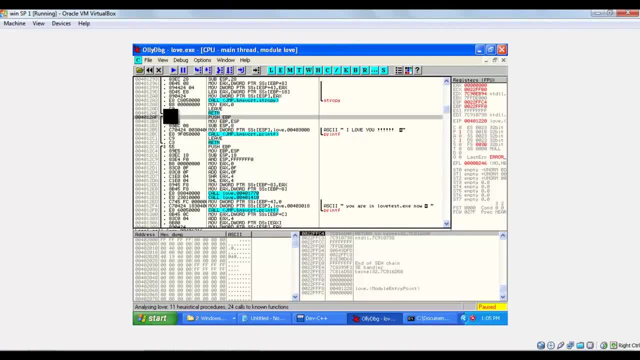 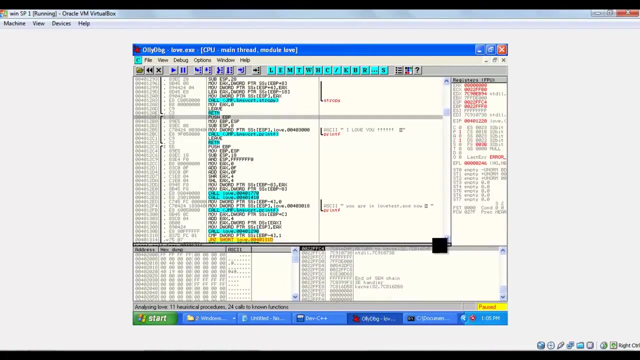 Now let us try to understand where we are actually getting a call to this, from where we are actually getting a call to this function. If you observe, I am just taking this function down. Oh, let me minimize. Let me minimize the window. 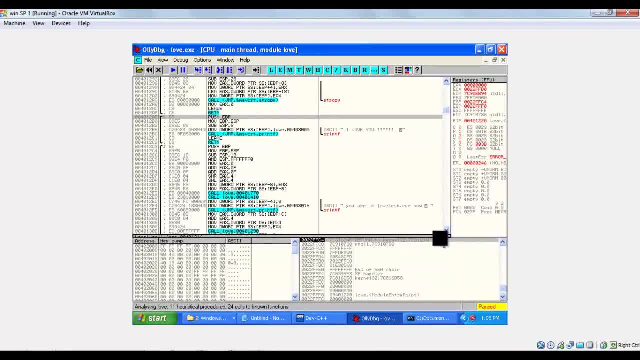 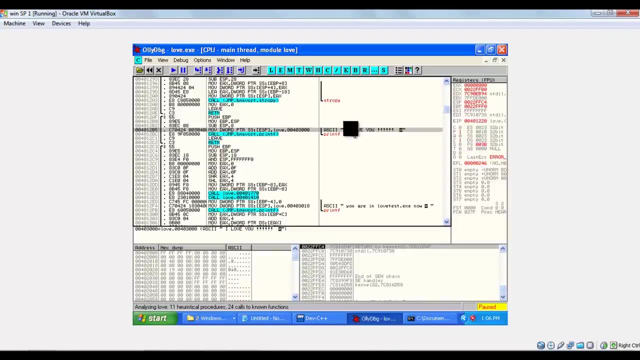 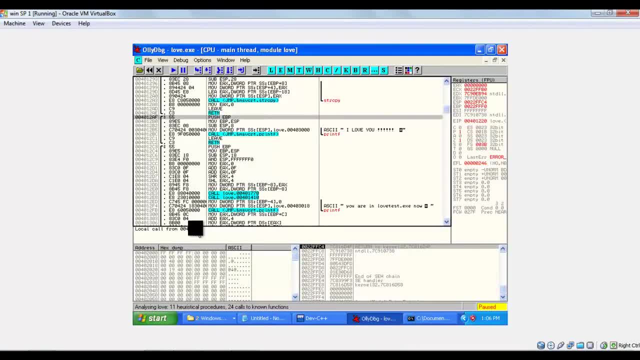 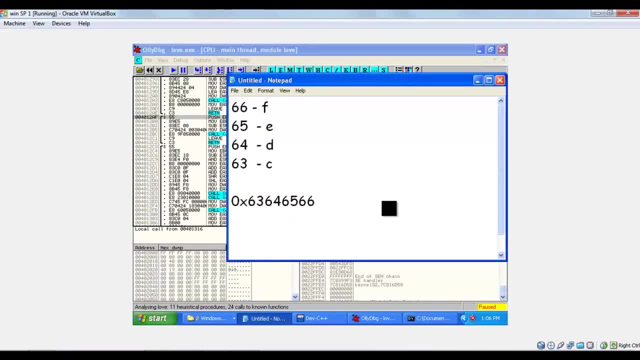 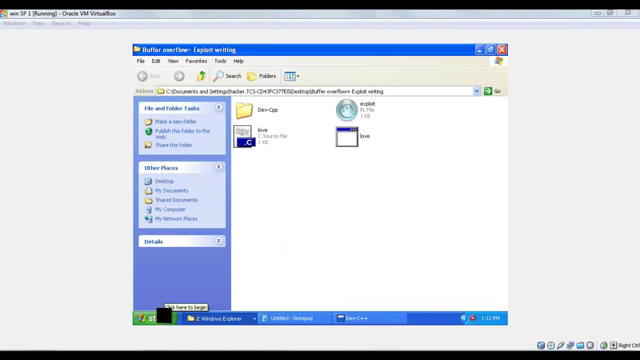 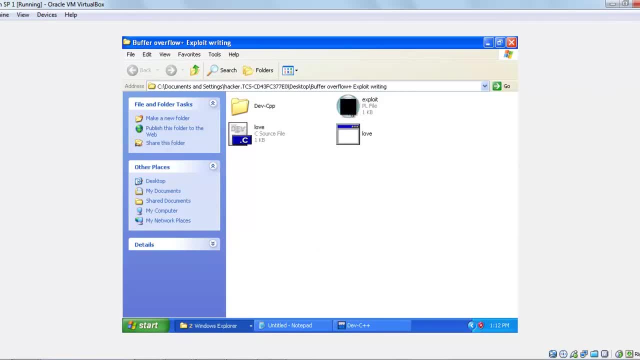 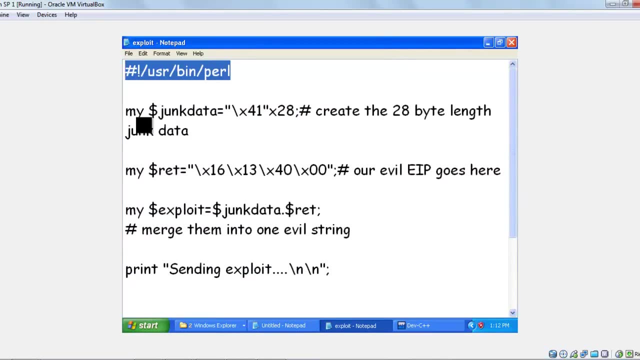 function and I am going to write a simple exploit in Perl language and see how it does. So this is a simple Perl script and in this I am taking a very simple variable which is actually taking 28 bytes of junk data, and this 41 represents capital A because this: 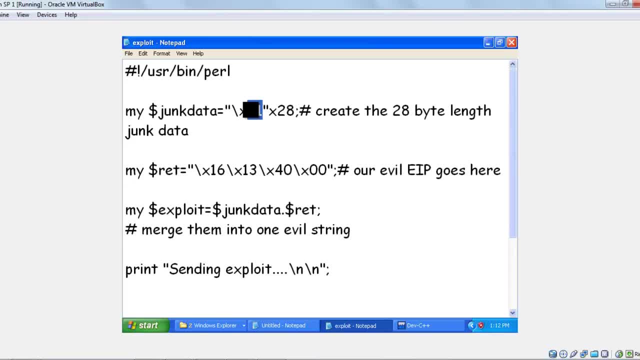 application is accepting 28 junk characters, so I am just going to give capital A of number 28.. And then I am going to give this evil EIP value to our exploit function and I am going to write a simple exploit in Perl language and see how it does. 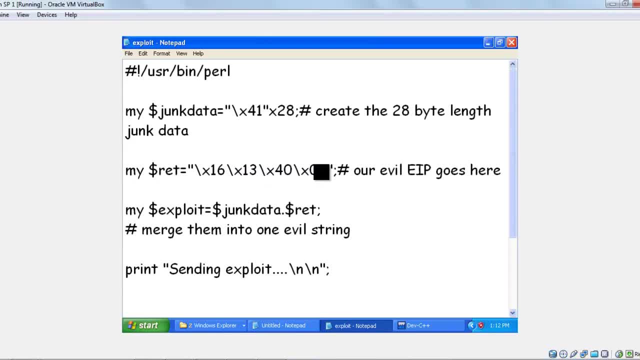 Now let us try to exploit the function by giving this evil EIP value to our exploit function and see how it does. So, this evil eip value which I have taken from my Olli dbg. this is the address of proposal of function. And now let us try to understand how we replaced, how we placed this address here. 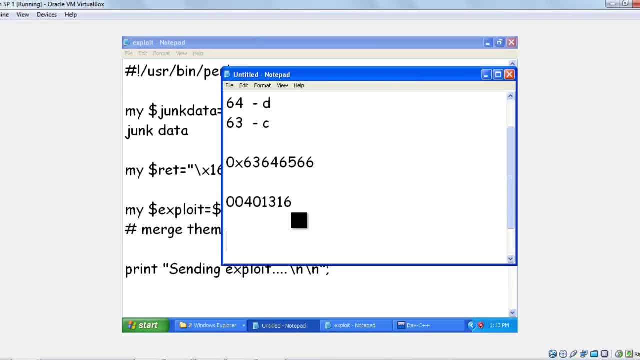 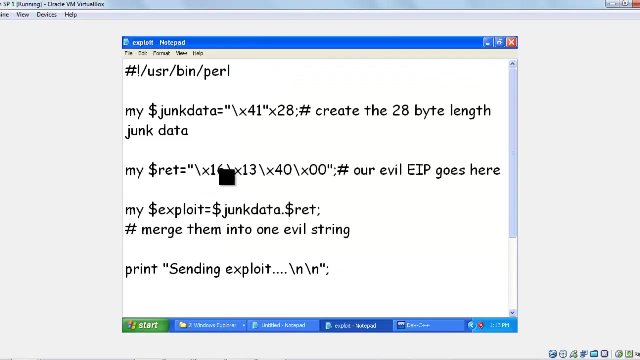 We have already noticed the address from Olli dbg over here, which is the function or proposal of address. Now, since it is in Bhaganian format, we have to convert it in to Lillianian format by putting, changing it to 1, 6, 1, 3, 4, 0 and 0: 0. now that's what we have placed. it placed. 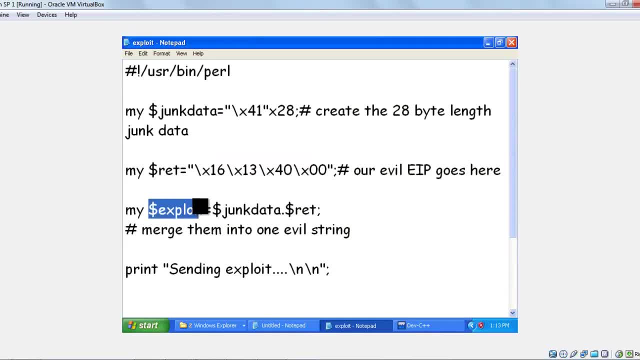 here and now we are taking one more variable and we are giving, we are assigning the value of junk data by appending this EIP value to that. now we are actually merging them into one evil string and we are giving it to the variable exploit. now we are printing, sending exploit. we'll see them, we'll see.